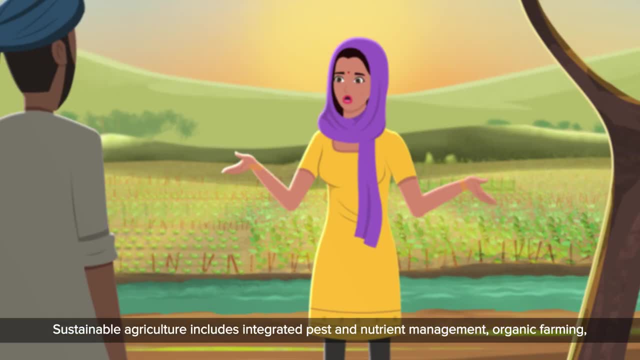 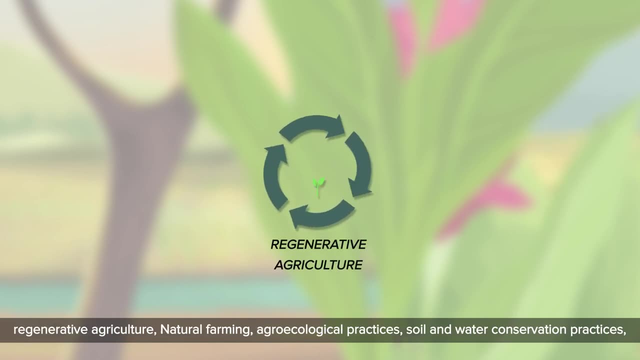 So how does it help us? Sustainable agriculture includes integrated pest and nutrient management, organic farming, regenerating agriculture, natural farming, agro-ecological practices, soil and water conservation practices, agroforestry, crop rotation and intercropping. 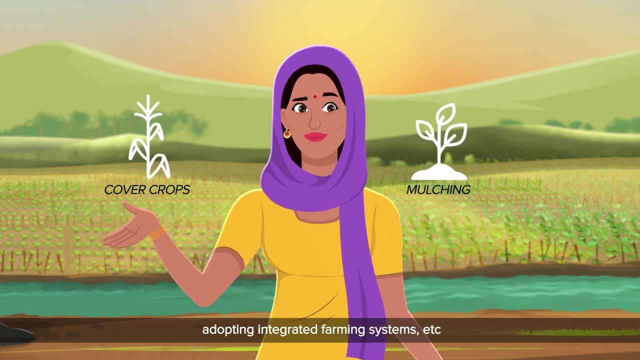 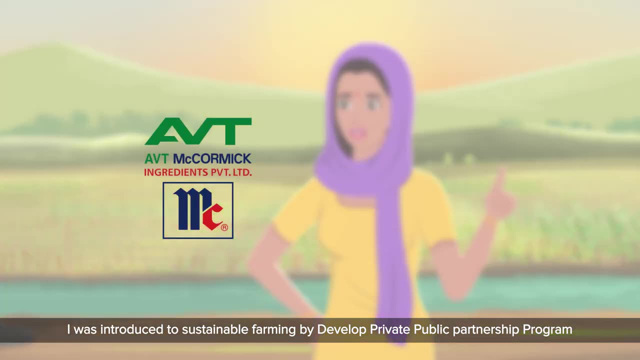 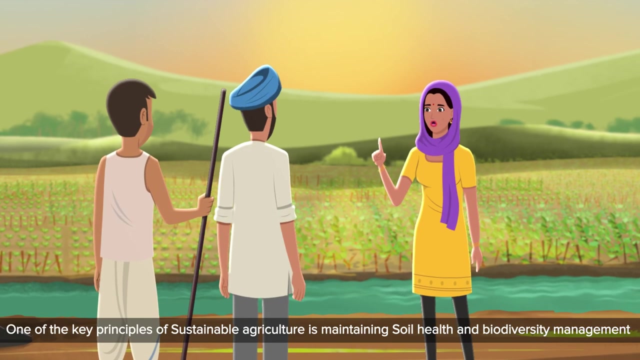 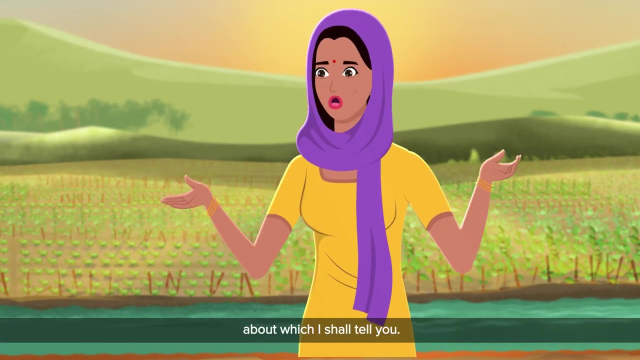 Using cover crops and mulching, and adopting integrated farming systems, etc. How do you know all this? I was introduced to sustainable farming by developed private-public partnership program initiated by AVT, Macomic and GIZ. One of the key principles of sustainable agriculture is maintaining soil health and biodiversity management, about which I shall tell you. 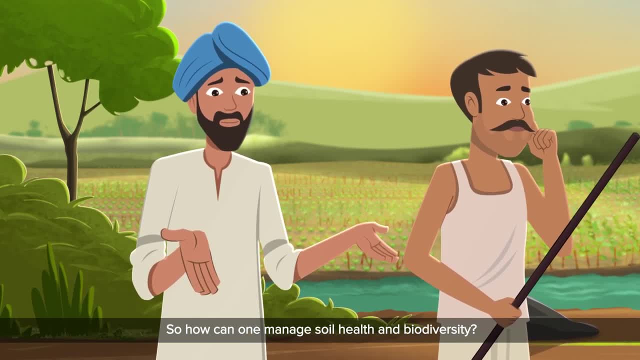 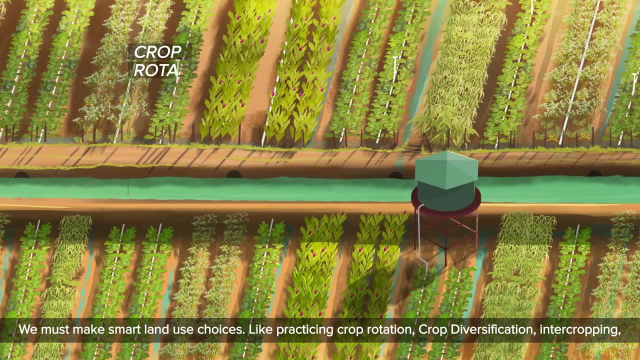 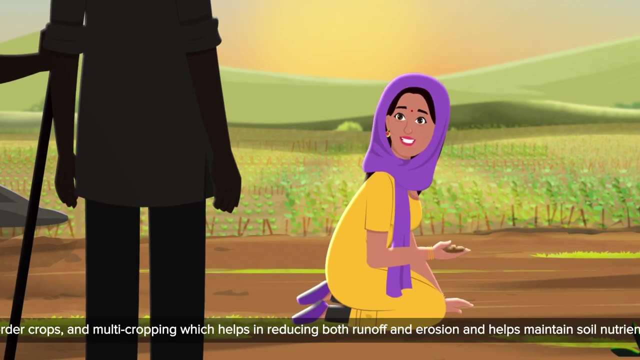 So how can one manage soil health and biodiversity? Come, I will show you. We must make smart land use choices like practicing crop rotation, crop diversification, intercropping, border crops and multi-cropping, which helps in reducing both runoff and erosion and helps maintain soil nutrients. 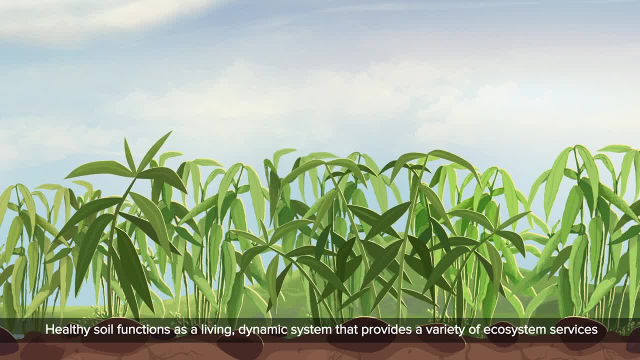 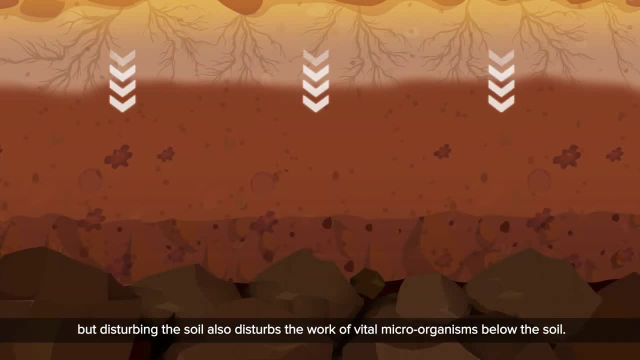 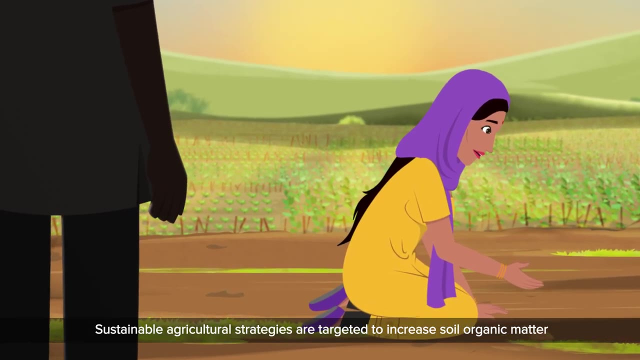 Healthy soil functions as a living dynamic system that provides a variety of ecosystem services. but disturbing the soil also disturbs the work of vital microorganisms below the soil. Then how do we turn this企業 into sustainable agriculture? Sustainable agricultural strategies are targeted to increase soil organic matter and reduce erosion through improvements in plant diversity and conservation tillage. 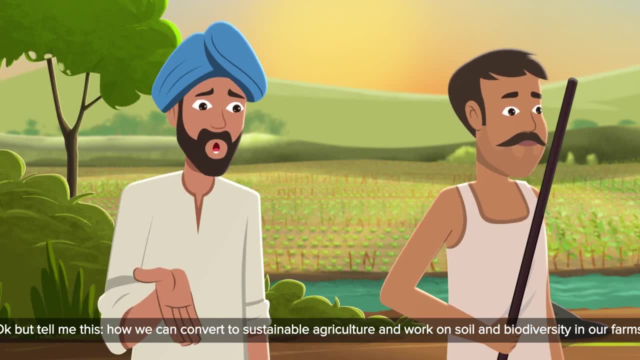 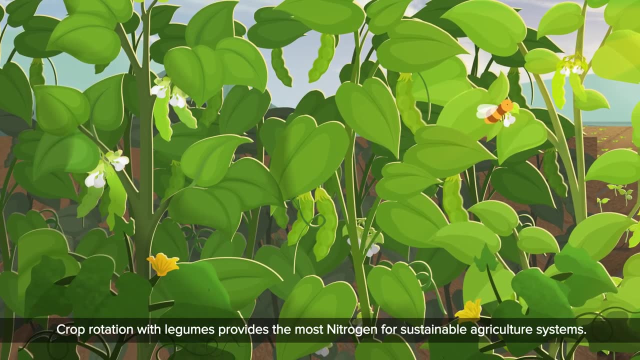 Okay, but tell me this: how can we convert to sustainable agriculture and work on soil and biodiversity in our farms? Listen carefully: Crop rotation with legumes provides the most nitrogen for sustainable agriculture systems. Conservation tillage practices: Conservation tillage purposes offers sustainable battling of Hofa, bear gear, animal Ocean, Kentucky and and many otherlardan tribal welfare systems. This involves bientôt70%слиwa Maheshwar пов cues, harato ke ina 둥, gestim cannons. management of bioisenca and farming practices. 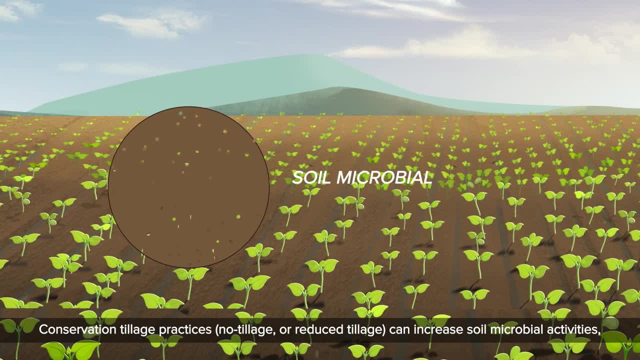 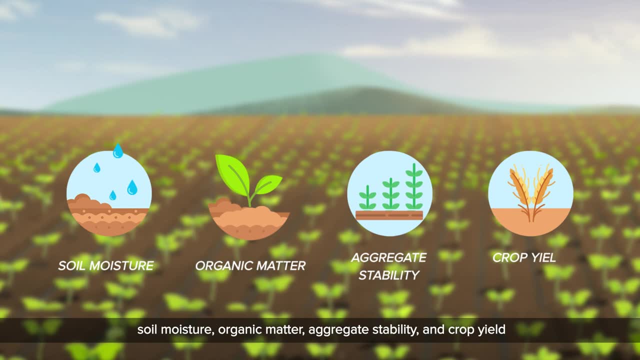 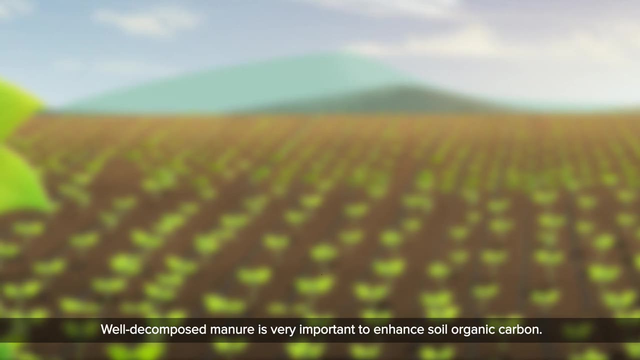 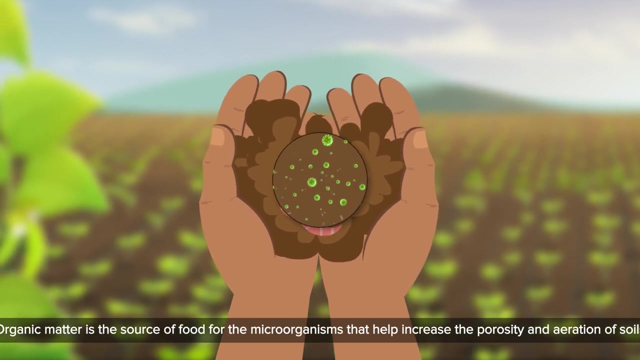 or reduced tillage can increase soil microbial activities, soil moisture, organic matter, aggregate stability and crop yield. soil organic carbon, that is, SOC, is extremely important for agriculture. well decomposed manure is very important to enhance soil organic carbon. organic matter is the source of food for the microorganisms that help increase the porosity and aeration of